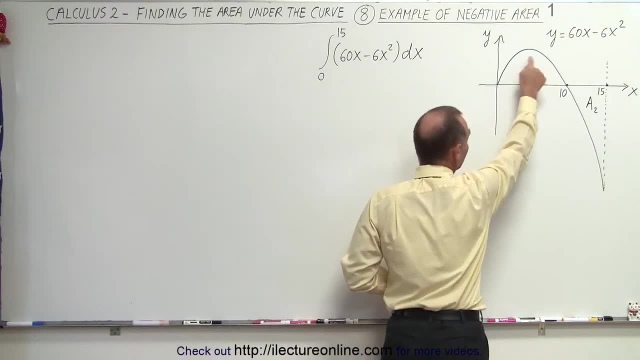 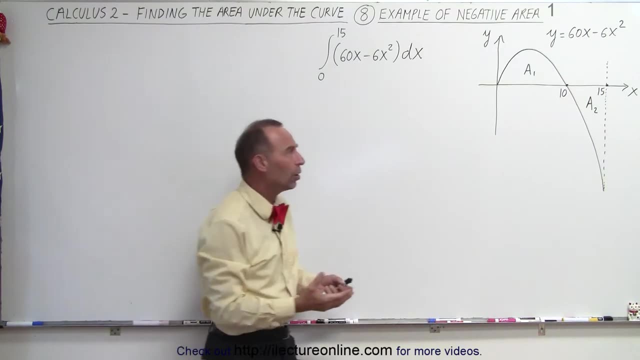 Well, it turns out that the area called a1 here in this drawing is indeed positive area and the area over here is indeed negative area, And sometimes we want to call this negative area and sometimes we want to look at that as being additional positive area. 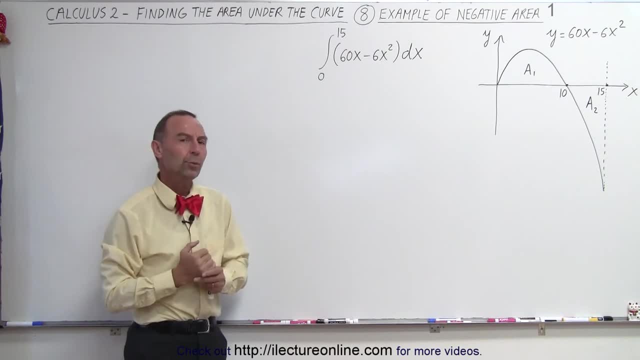 And so how do we know the difference? When do we use one, When do we use the other? Well, let's first understand what the concept of negative area is by solving this particular integral. Let's say that someone asks you to find the area underneath the curve defined by. 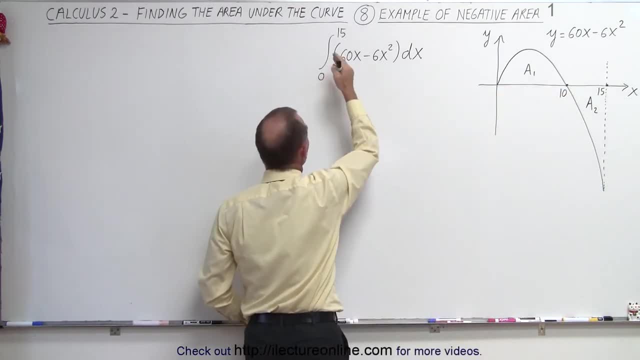 this equation right there, and the limits of integration are from 0 to 15.. And if you did not draw out the curve, if you did not know what that looked like, and you went ahead. and if you did not draw out the curve, if you did not know what that looked like, 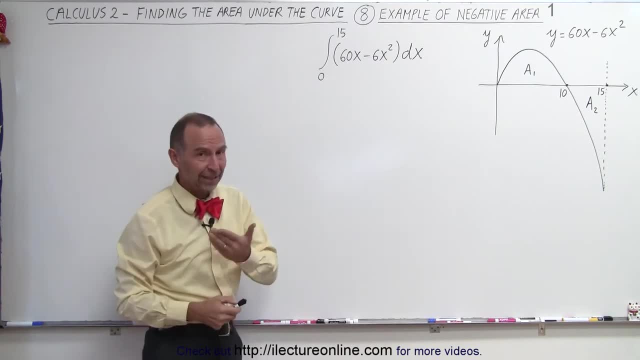 and if you did not draw out the curve, if you did not know what that looked like and tried to find the area underneath the curve? well, let's see what would happen if we did just that. So first we're going to integrate this, So this becomes equal to 60. 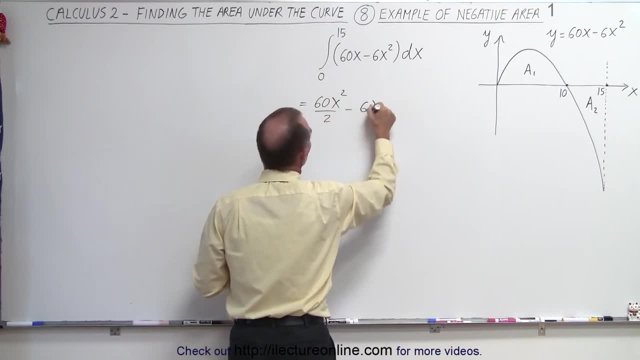 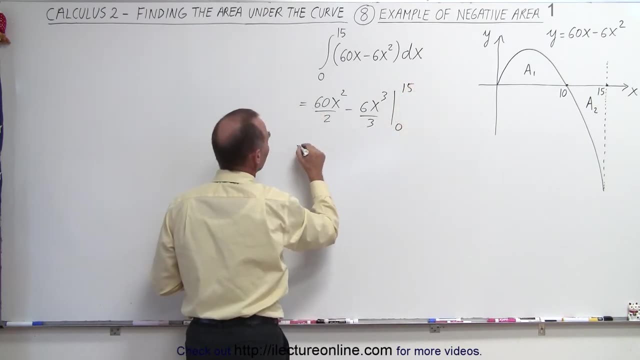 x squared divided by 2, minus 6 x cubed divided by 3, evaluated from 0 to 15. And of course we can simplify that a little bit. This becomes equal to 30 x squared minus 2 x cubed from 0 to 15.. And of course, when we plug in the lower limit, we don't get anything. 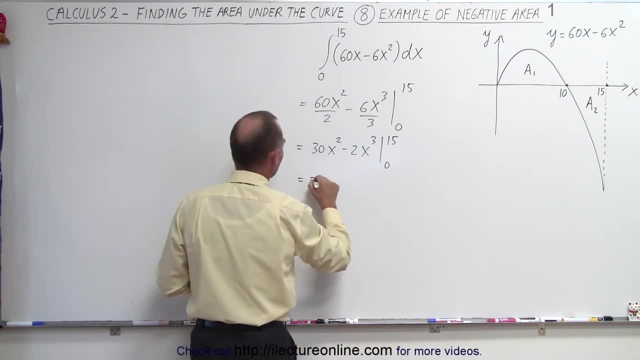 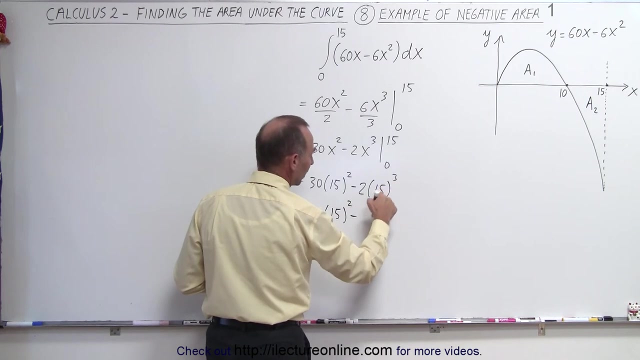 When we plug in the upper limit, we get the following: This is equal to 30 x 15 squared minus 2 x 15 cubed. Well, when you work that out, this is equal to 30 x 15 squared minus. if I take one of these 15's. 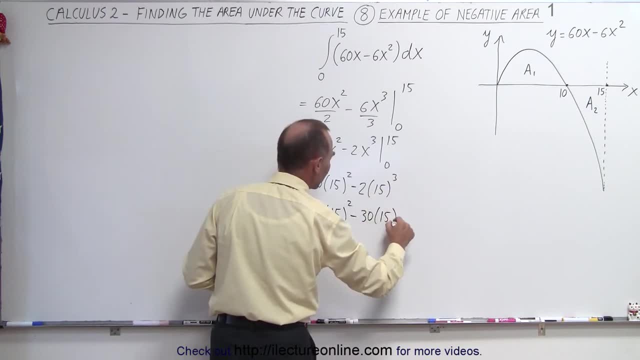 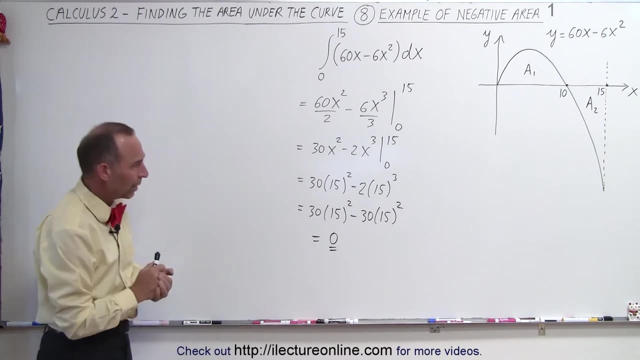 multiply times 2, I get 30 x 15 squared And notice that is exactly equal to 0.. And so you'd be kind of perplexed and go: wow, that's zero. How can that be? How can the area need a curve be zero? Well, once we draw it out, we 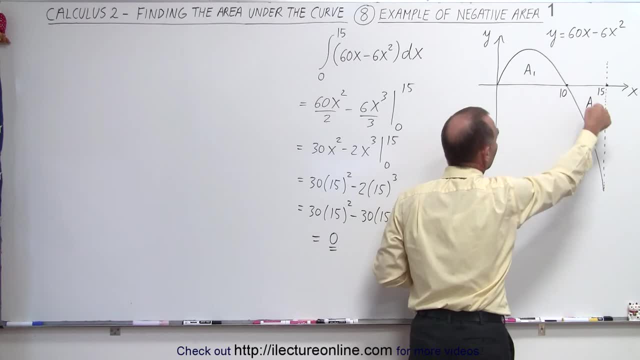 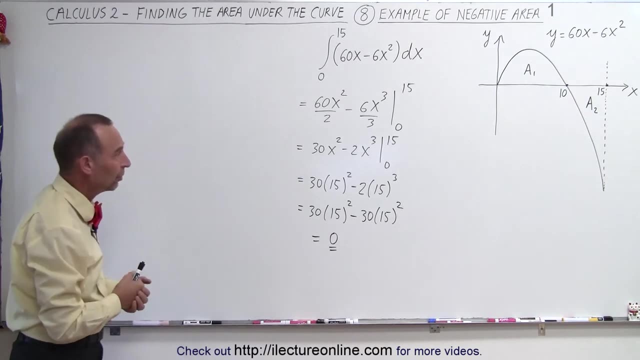 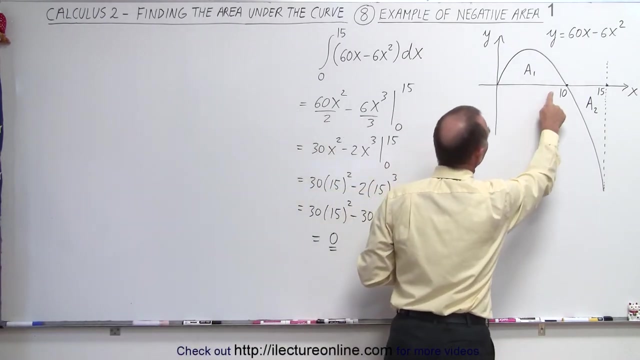 probably realize that a1, being positive area, and a2 being negative area, are probably equal in size and they cancel each other out and therefore the net area is equal to zero. To show that that's true, let's go ahead and do two separate integrals. We first are going to integrate from 0 to 10. 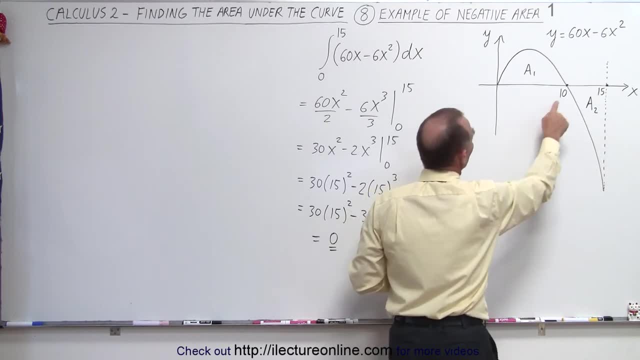 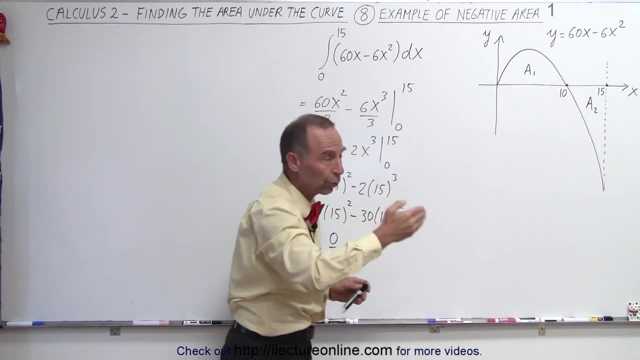 and then from 10 to 15 and see what we get in each case. Notice that if you plug in 10 for x, we get minus 600, which is 0. That means that's the point where the curve crosses the x-axis. So let's go. 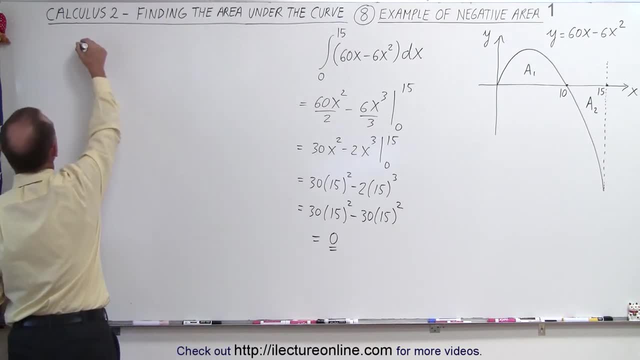 ahead and integrate the integral from 0 to 10 and see what we get. So the integral from 0 to 10 of the quantity 60 x minus 6 x squared dx is equal to well, that would be equal to 60 x squared divided. 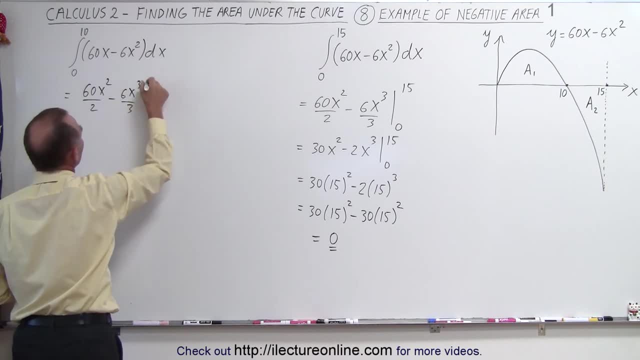 by 2 minus 6 x cubed, divided by 3, from 0 to 10.. So that's equal to 30 x squared minus 2 x cubed from 0 to 10. and those limits are easy to plug in. Notice, when we plug in 0, we get nothing. Plug in 10, we get. let's see, that's 100 times 3, that's 3000. 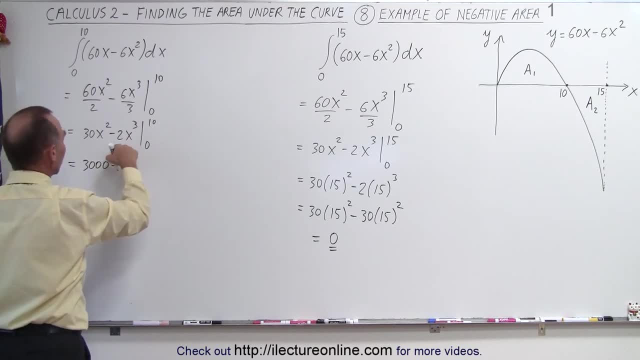 minus that would be a hundred. that would be a thousand times two minus two thousand. Notice that is equal to one thousand, which means the area underneath the curve going from 0 to 10 is equal to one thousand. Let's see what we get when we integrate the second. 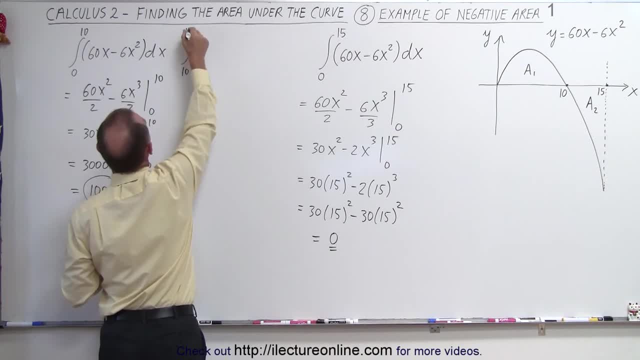 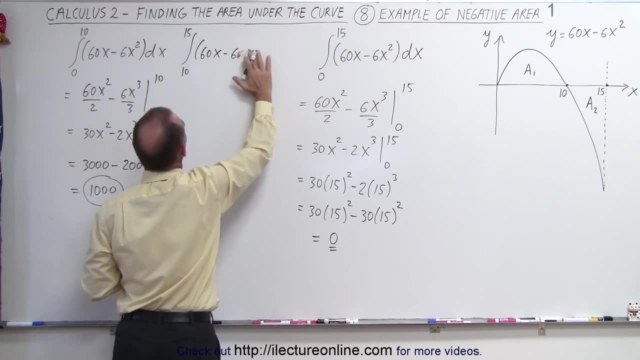 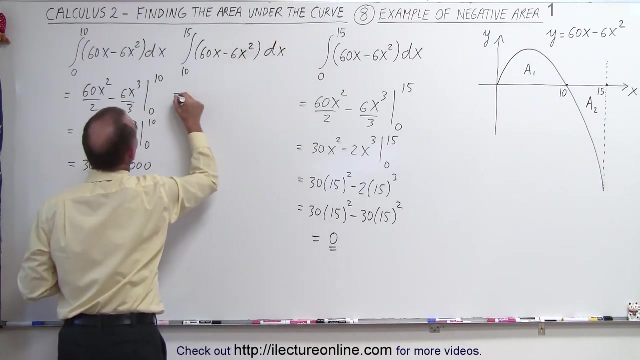 one. So now we're going to integrate from 10 to 15 the same integral: 60 x minus 60 x, not 60, but 6 x squared. That's kind of a mess: 6 x squared times dx. and again, by now you realize that this is equal to. 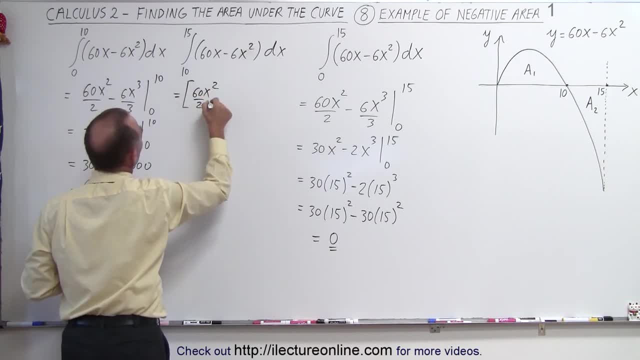 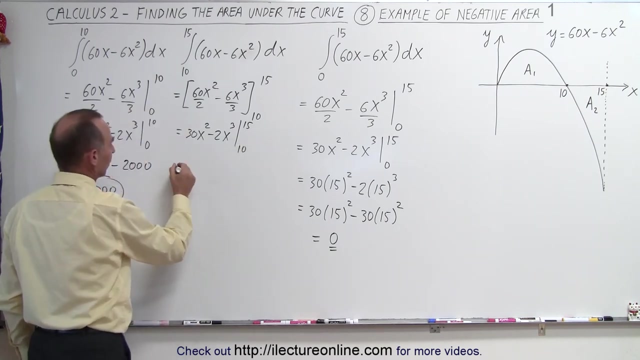 60 x squared over 2.. over 2 minus 6 x cubed, over 3, going from 10 to 15 this time, and so this is equal to 30 x squared minus 2 x cubed, evaluated from 10 to 15.. So when I plug in the limits, see what we get. so this: 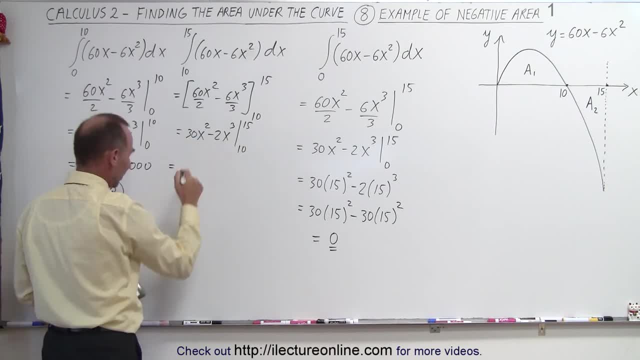 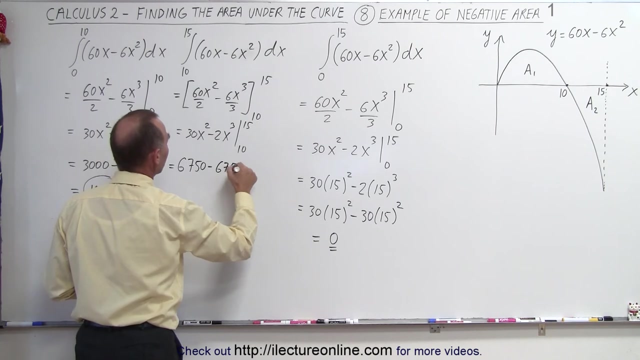 becomes equal to 30 x 15 squared. so let's see: 15 squared x 30. that gives us 6750 minus and, just like what we realized here, that's going to be the same. so that's going to be 6750. that's for the 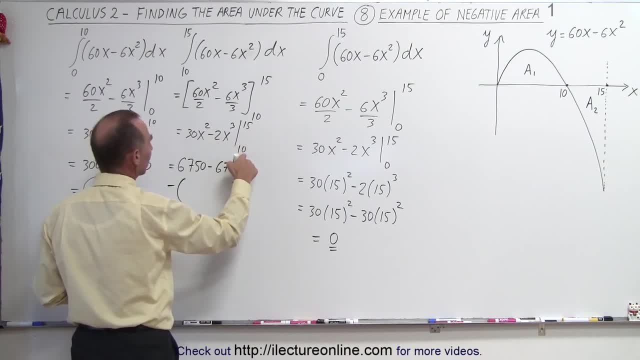 upper limit minus when we plug in the lower limit. so we plug that in here, we get 100 times that, that's 3000. minus plug in the limit there, that's a thousand times two, that's 2000. but notice it's subtracted so we get zero minus a thousand. this is equal to a minus thousand. 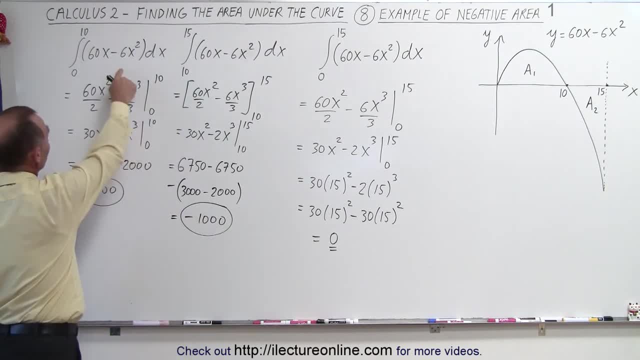 and sure enough, we realize now that a1, which is defined by this integral right here, is equal to a thousand, and a2, which is defined by this integral right here, becomes minus a thousand, and when you add the two together you do indeed get zero. So you can see here that you always have 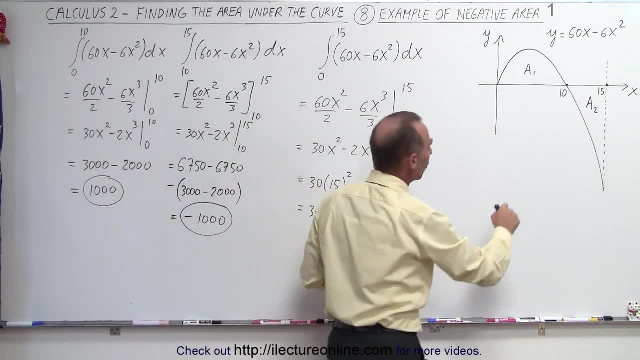 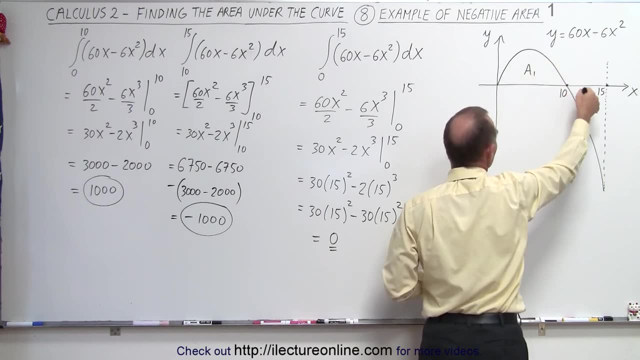 to be careful about positive and negative area, that you have to understand where the curve crosses the x-axis. you have to understand that you need to put the limits from there to there if you want to just get the positive area and from there to there when you just want to get the negative area and when 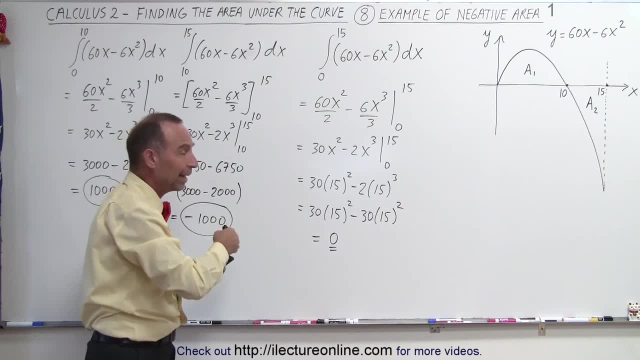 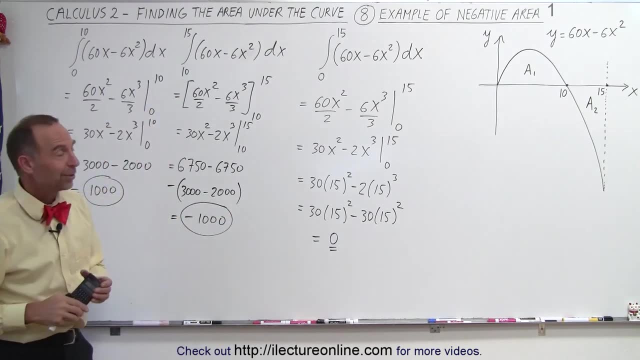 you simply want to get the total area and you want to combine the positive and the negative area together, then of course you can integrate from 0 to 15, and in this case the answer will indeed be 0.. So that gives you hopefully a better understanding of what we mean by positive and. 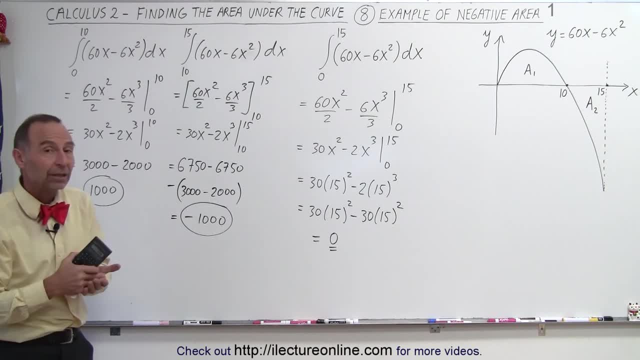 negative area, and we're going to do a few more videos where we can explain why we care and why sometimes the negative area does indeed indicate something and why sometimes we do want to consider the negative area as positive area. So you'll see in just a moment in some other videos how that's.